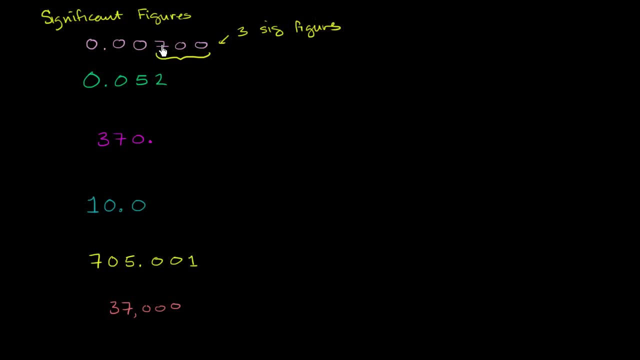 And that is true, but there's not. it's not telling us how precise our measurement is. And to try to understand this a little bit better, imagine if this right over here was a measurement of kilometers. So if we measured 0.00700 kilometers, that same measurement we could have. this would be the exact same thing as 7.00 meters. 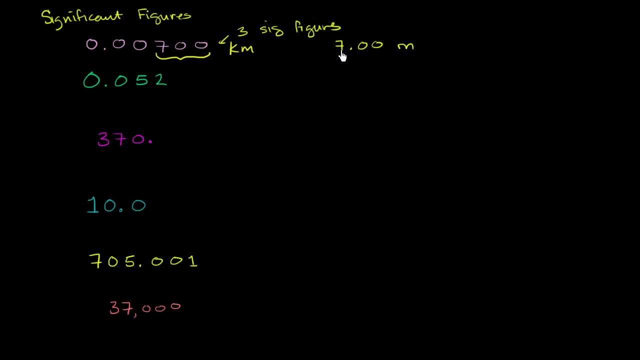 Maybe. In fact we just used a meter stick and we said it's exactly 7.00 meters. So we measured to the nearest centimeter And we just felt like writing it in kilometers. These two numbers are the exact same thing. 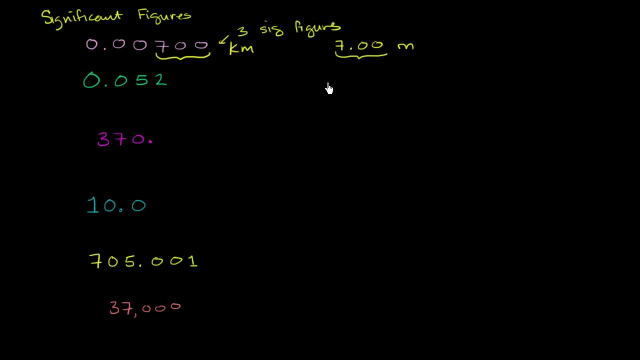 They're just different units. But I think when you look over here it makes a lot more sense why you only have three significant figures. These zeros are just kind of telling. you are just shifting it based on, maybe what the units of measurement that you're using. 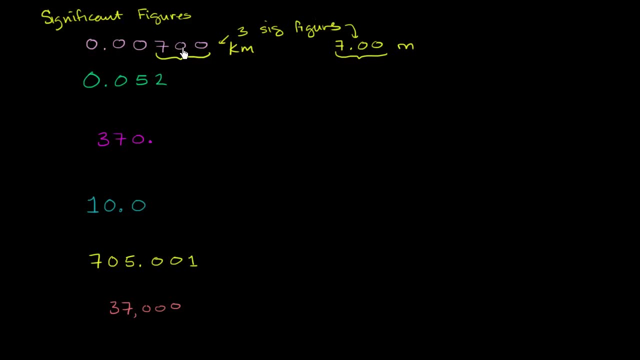 But the numbers that are really giving you the precision are the 7, the 0. And the 0. And the reason why we're counting these trailing zeros is that you didn't. whoever wrote this number didn't have to write them down. 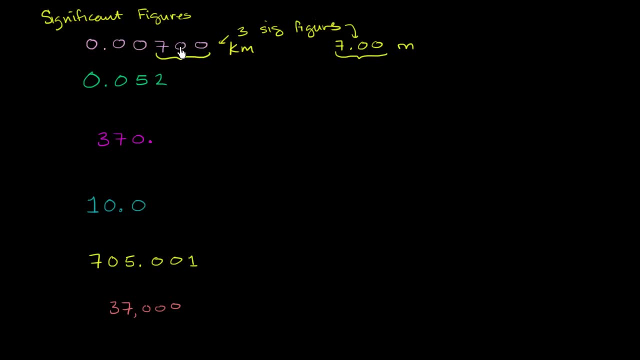 They wrote them down to explicitly say: look, I measured this far. If they didn't measure this far, they would have just left these zeros off and they would have just told you 7 meters, not 7.00.. Let's do the next one. 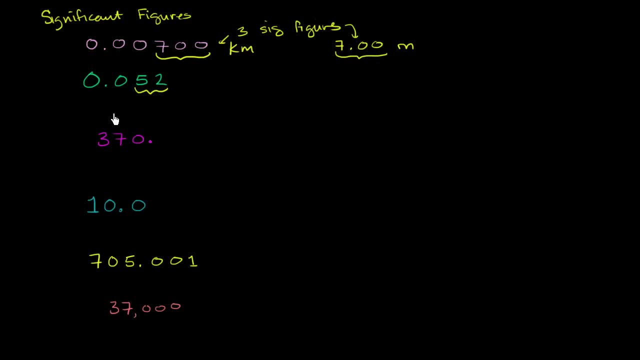 So, based on the same idea, we have the 5 and the 2, the non-zero digits are going to be significant figures. You don't include this leading zero, by the same logic That if this was 0.00.. 5, 2 kilometers, this would be the same thing as 52 meters, which clearly only has two significant figures. 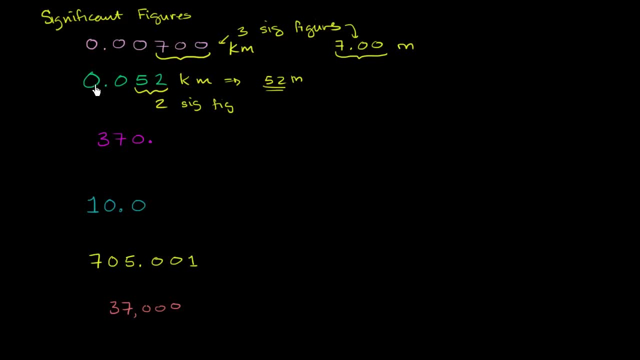 So you don't want to count leading zeros that are leading zeros before the first non-zero, before the first non-zero digit. I guess we could say You don't want to include those, You just want to include all the non-zero digits. 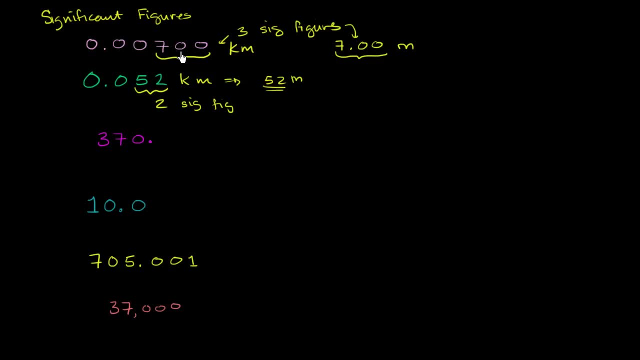 And everything in between, And trailing zeros. trailing zeros if a decimal point is involved. I'll make those ideas a little bit more formal. So over here the person did 370, and then they wrote the decimal point. If they didn't write the decimal point, it would be a little unclear on how precise this was. 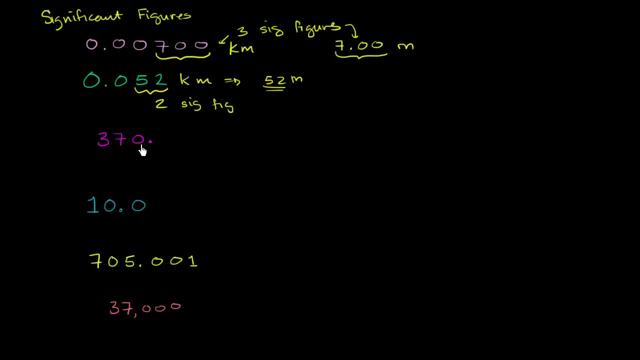 But because they wrote the decimal point, it means that they measured it exactly to be 370.. They didn't get 372 and then round down or they didn't have kind of a roughness, only to the nearest tens place. They didn't get 372 and then round down or they didn't have kind of a roughness, only to the nearest tens place. 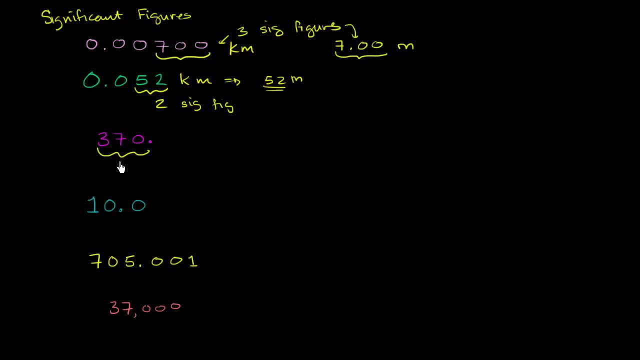 This decimal point is going to be 370.. This decimal point is going to be 370.. This decimal tells you that all three of these are significant. So this is three significant figures over here. Then on this next one, once again, this decimal tells us that not only did we get to the nearest one, 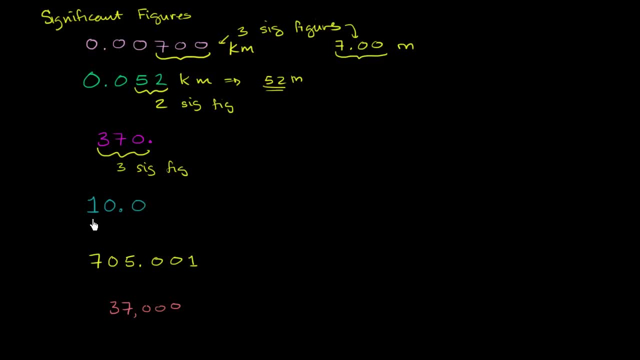 but then we put another trailing zero here, which means we got to the nearest tenth. So in this situation, once again we have three significant figures Over here. the seven is in the hundreds, but we got all the way down. The measurement went all the way down to the thousandths place. 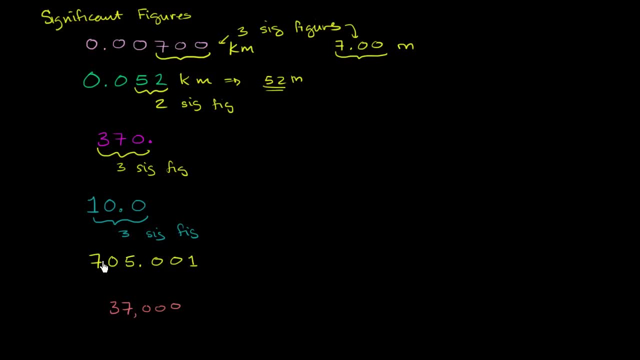 Even though there are zeros in between. those zeros are part of our measurement because they are in between non-zero digits. So in this situation, every digit, every digit here, the way it's written, is a significant digit. So you have six significant digits. 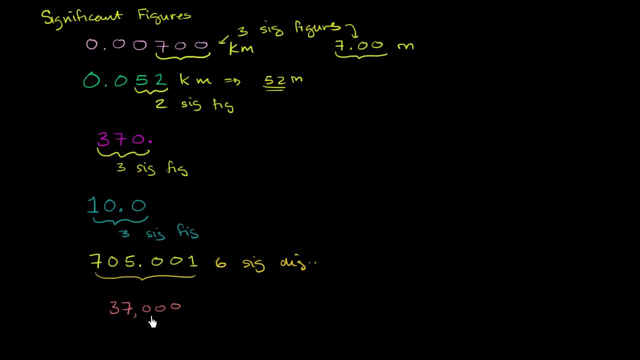 Now this last one is ambiguous: The 37,000, it's not clear whether you measured exactly 37,000.. Maybe you measured to the nearest one and you got an exact number. You got exactly 37,000. Or maybe you only measured to the nearest thousand. 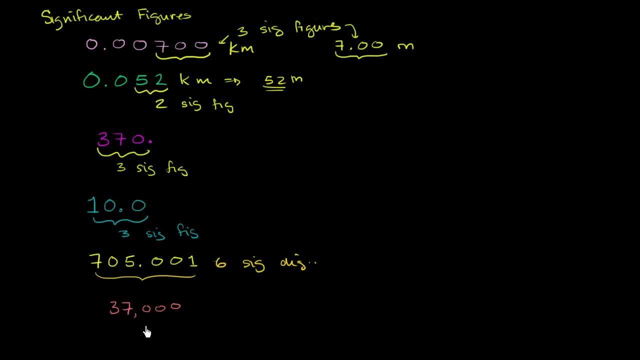 So it depends on what you know. there's a little bit of ambiguity here. If you just see something written exactly like this, you would probably say, if you had to guess or not guess, if there wasn't any more information, you would say that there's just two significant digits. 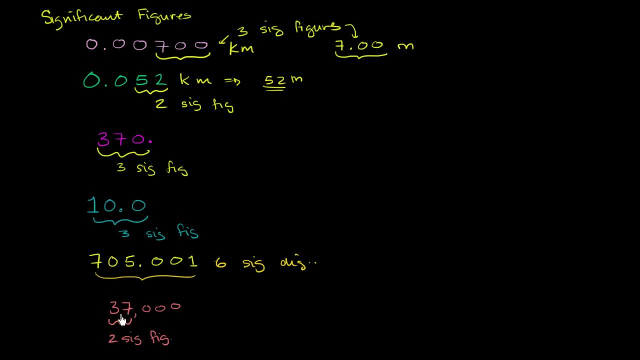 Two significant figures or two significant digits For this person- to be less ambiguous, they would want to put a decimal point right over there- And that lets you know that this is actually five digits, Five digits of precision, That we actually go to five significant figures. 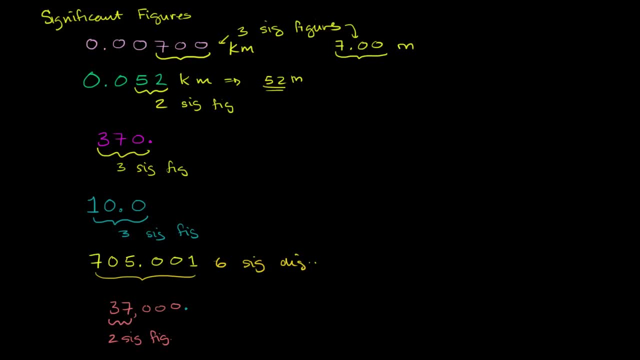 So if you don't see that decimal point, I would go with two.